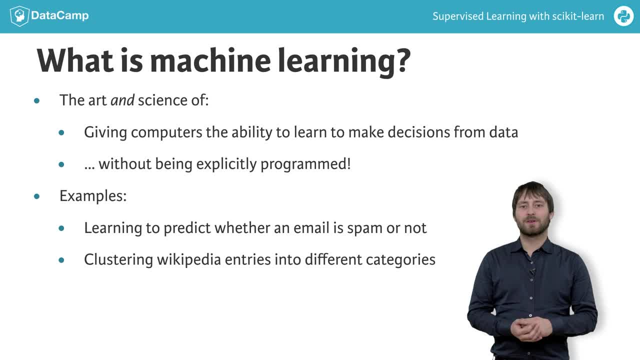 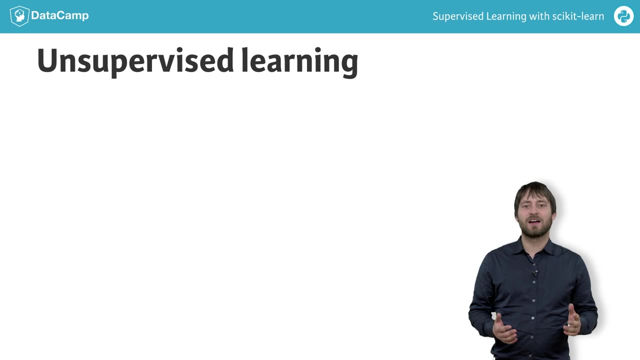 In the second example there is no such label. When there are labels present, we call it supervised learning. When there are no labels present, we call it unsupervised learning. Unsupervised learning, in essence, is the machine learning task of uncovering hidden patterns. 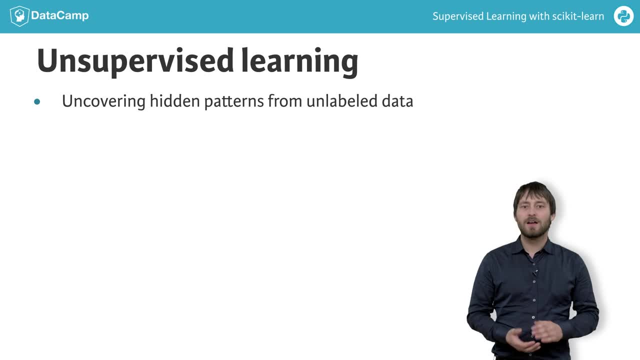 and structures from unlabeled data. For example, a business may wish to group its customers into distinct categories based on their purchasing behavior, without knowing in advance what these categories might be. This is known as clustering, one branch of unsupervised learning. 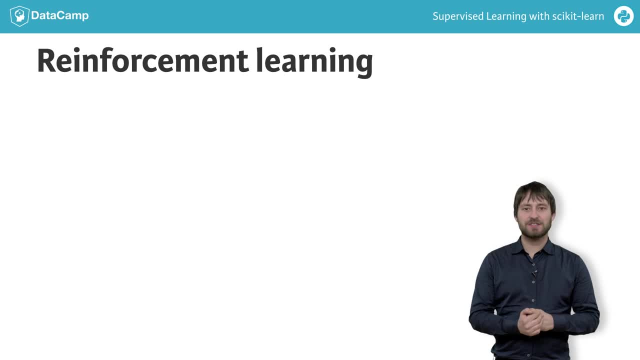 There is also reinforcement learning, in which machines or software agents interact with an environment. Reinforcement learning agents are able to automatically figure out how to use the environment, how to optimize their behavior, give them a system of rewards and punishments. Reinforcement learning draws inspiration from behavioral psychology and has applications in many fields. 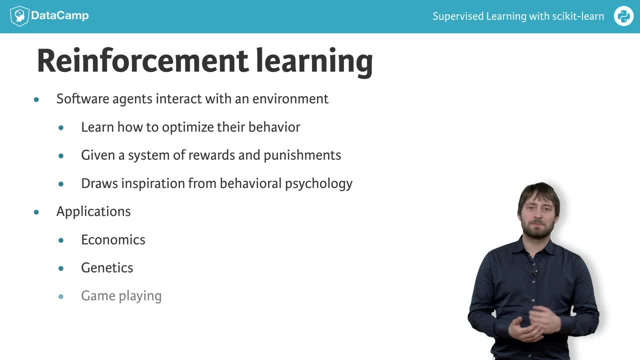 such as economics, genetics, as well as game playing. In 2016,, reinforcement learning was used to train Google DeepMind's AlphaGo, which was the first computer program to beat the world champion in Go. But let's come back to supervised learning, which will be the focus of this course. 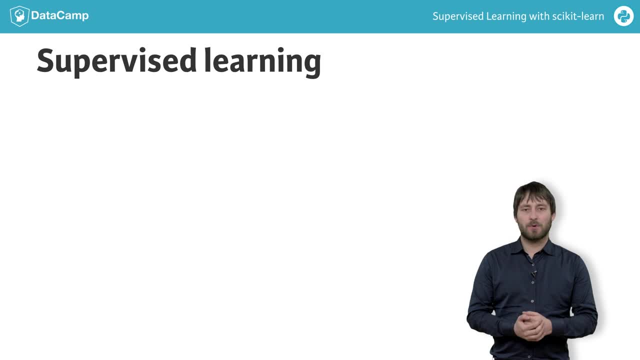 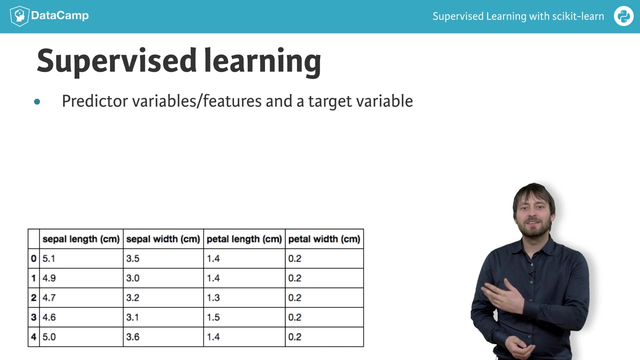 In supervised learning, we have several data points or samples, described using predictive variables or features and the target variable. Our data is commonly represented in a table structure such as the one you see here, in which there is a row for each data point and a column for each feature. 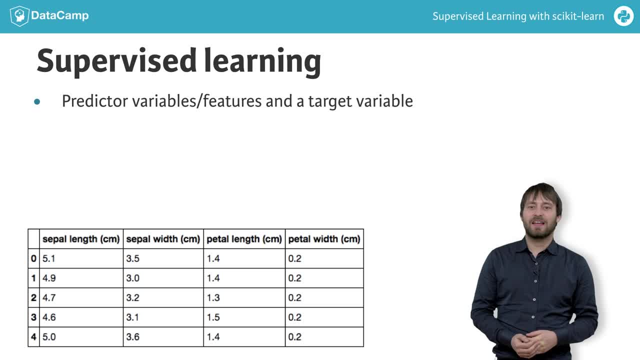 Here we see that. You see the IRIS dataset. Each row represents measurements of a different flower and each column is a particular kind of measurement, like the width and length of a certain part of the flower. The aim of supervised learning is to build a model that's able to predict. 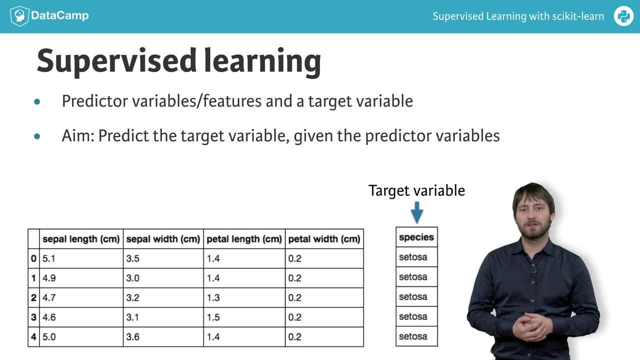 the target variable, here the particular species of the flower. given the predicted variables- here the physical measurements. If the target variable consists of categories like click or no, click spam or not spam, or different species of flowers, we call the learning task.